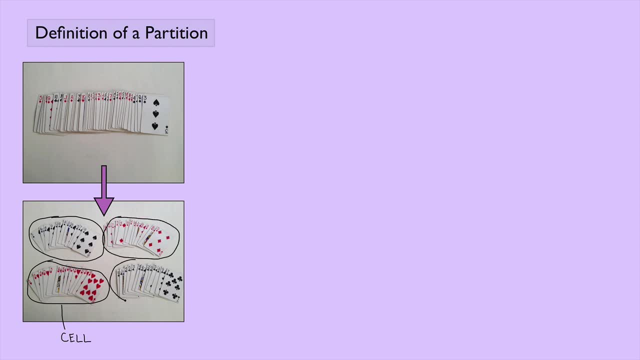 cell, and this would be another cell, and this would be another cell. And so we've taken the set of cards, and we've partitioned it into four different cells. Another example, suppose you 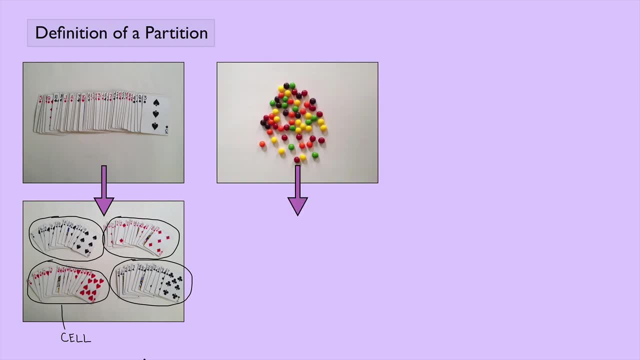 have a set of hearts, and you're partitioning it into four different subsets. And so you're going to have a set of delicious candies. You could, if you wanted to, sort the delicious candies by color. So we've partitioned the set of candies here, and we would have, in this case, five different cells. Each of these is a cell. And you might see some books refer to each of these as classes as well, but I'm going to use the word cell because class ends up meaning something else later on. So each of these things would be a cell. Okay, so what do we notice here? Well, 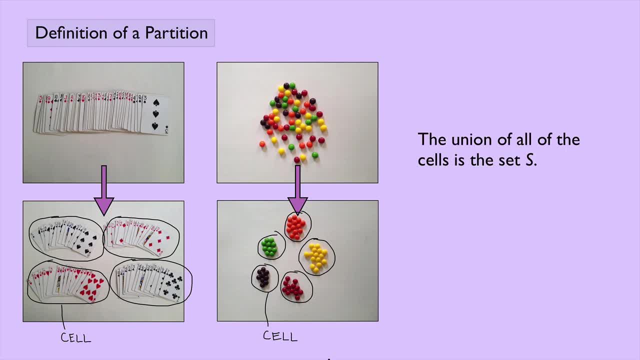 we see that the union of all the cells is the set S. In other words, here's our set of candies. We could call that the set S. And the union of the cells, that means you just take all the cells together. That would be the same thing as the set of the candies we started with. 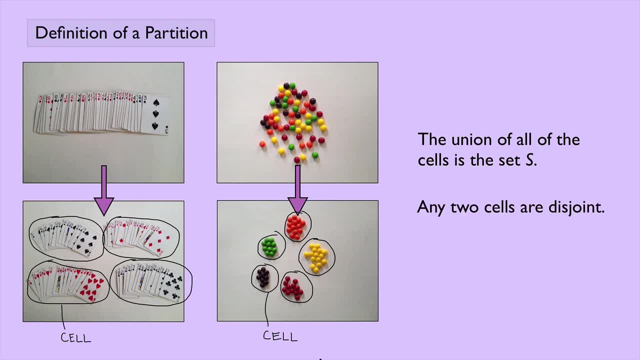 Another thing we see is that any two cells are disjoint. Look at the, say, the orange candies and the yellow candies. There are no candies, orange candies in the yellow set, and there are no yellow candies in the orange set. In other words, these two cells are separate from each other. There's no overlap here. And that's true of any two cells that you take. They are disjoint. 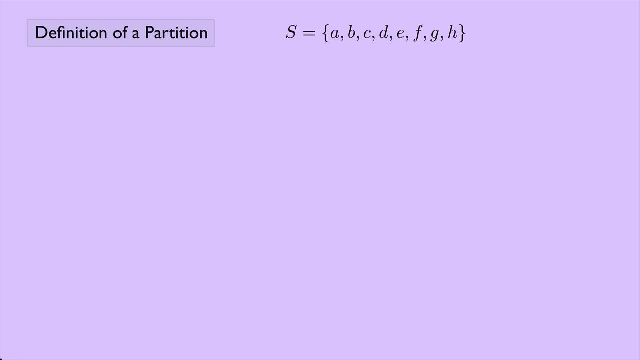 That's what that word means. So let's look at another example. Suppose we have the set S, which has the elements A, B, C, D, E, F, G, and H. And we can make a partition by saying, 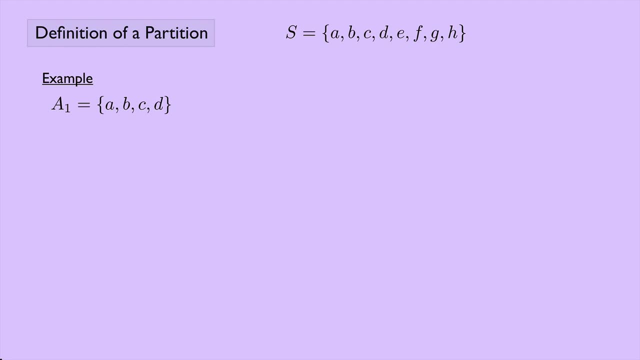 well, I'll call one of the cells A1. That would be A, B, C, and D. And we could have another cell, A2, which we could call E, F, G, and H. And notice that if you take the union of A1 and A2, that you get S, and that these two cells are disjoint. Here's another example. Suppose A1 is A, C, and G. A2 is disjoint. Here's another example. Suppose A1 is A, C, and G. A2 is disjoint. 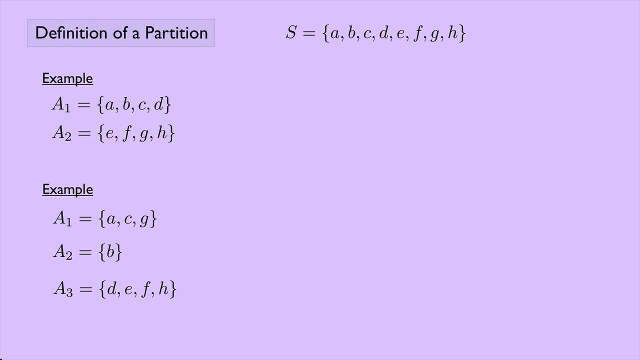 Just the element B. And A3 is D, E, F, and H. If we look at this, we see that every element of S is in one of these three cells. And we see that the cells are disjoint. So really, there's two 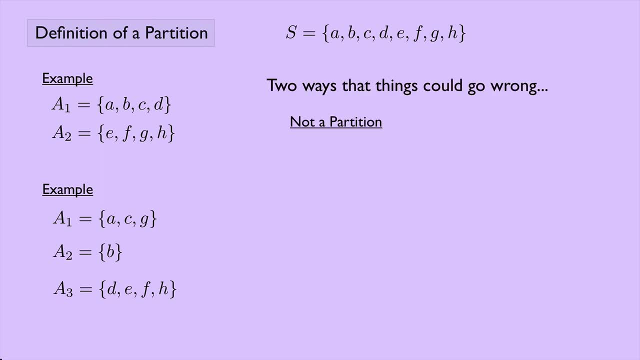 ways that things could go wrong. We could have something like this. So this is not a partition. 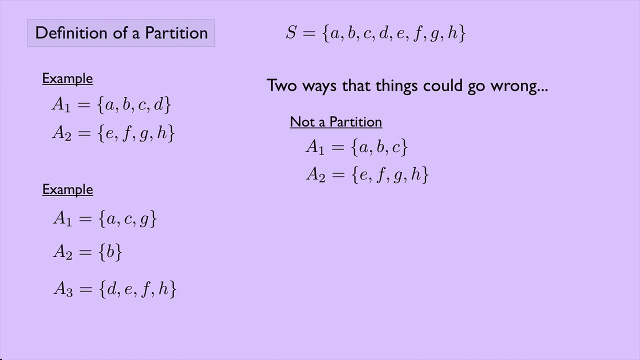 A1 is A, B, and C. A2 is E, F, G, and H. What's the problem here? Well, there's no disjoint. So we could have something like this. So we could have something like this. 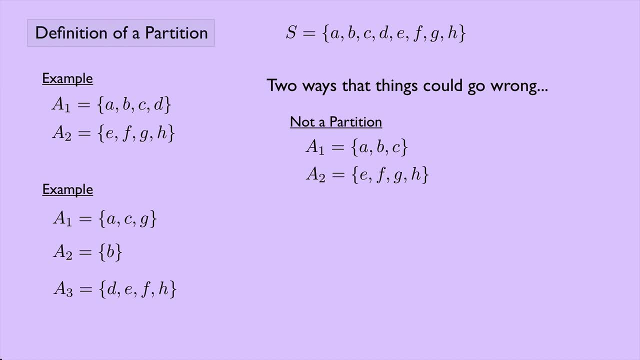 We could have D. And remember, if we take the union of the cells, it means to take them all together, we should get the set S. In this case, we wouldn't. We'd be missing D. So that's not a 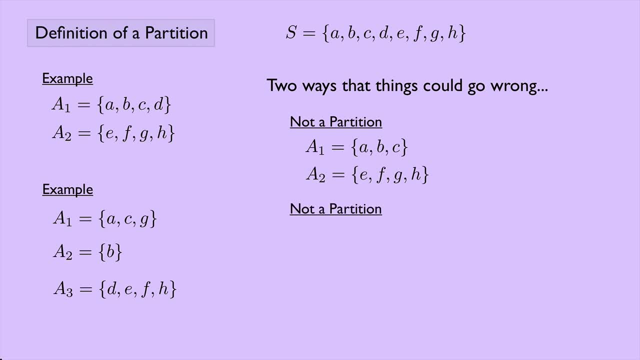 partition. Here's another thing that's not a partition. Suppose we have A1 is A, B, and C. A2 is C, D, E, F, G, and H. Well, now if we take the union of A1 and A2, we do indeed get the set S, but we have a problem. The cells are not disjoint. We can see here that this element C 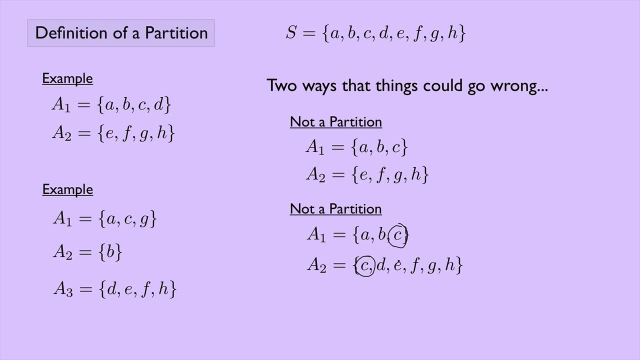 shows up in two different cells, A1 and A2. So that's not a partition. 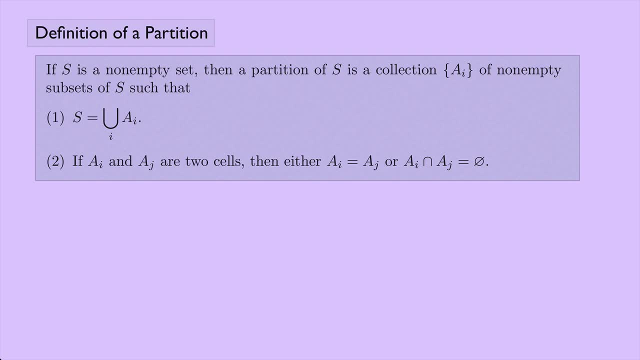 All right, I think it's time for the actual definition. If S is a non-empty set, then a partition of S is a collection, and we can call those A sub I, the index I will indicate which cell we're talking about, of non-empty subsets of S such that, and these were the two conditions. So remember before we had the two things, two ways things could go wrong. So, these two conditions kind of take care of that. Condition one says that the set S is the union of all of the cells. So this big U here means the union, and over the index I here, and so we would add up A1 and A2 and A3 and A4. You take all the cells together. That should give you the set S. And condition two, we have if A I and A J are two cells, then either, well, they're the same cell or they're completely disjoint. That means you take the intersection of them and you get the empty set. There's no overlap between them. So that kind of makes sense. We know that either they're the same cell or they're completely separate from each other. Okay, let's look at